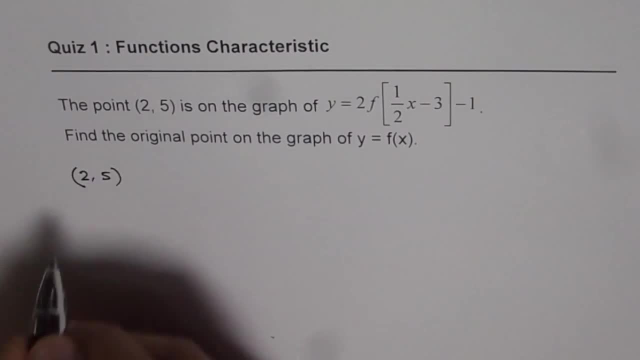 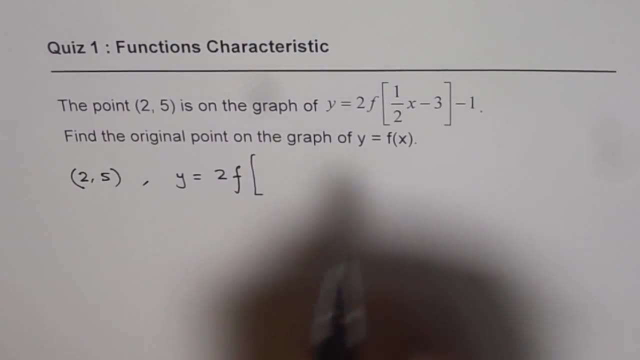 So we are given the point which is, and it is on the function, y equals to 2 times f of. now it is good to always factor half right, so we have half x minus 6 minus 1.. Now this is a transform function of y equals to f of x. We have to find the point on the. 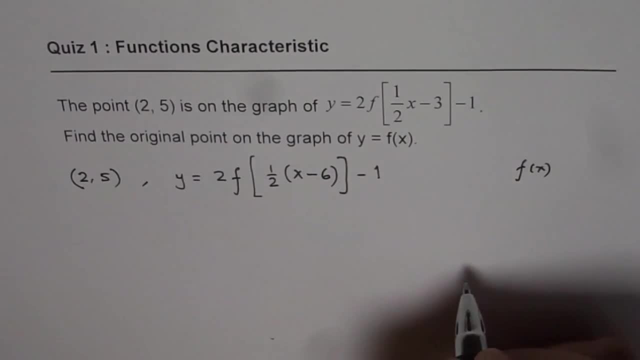 original function: f of x. right, that is the whole idea. So this point 2, 5 is on the given function. Let the point on f of x be x, 2,, 3,, 4,, 5,, 6,, 7,, 8,, 9,, 10,, 11,, 12,, 13,, 14,, 15,, 16,, 17,, 18,. 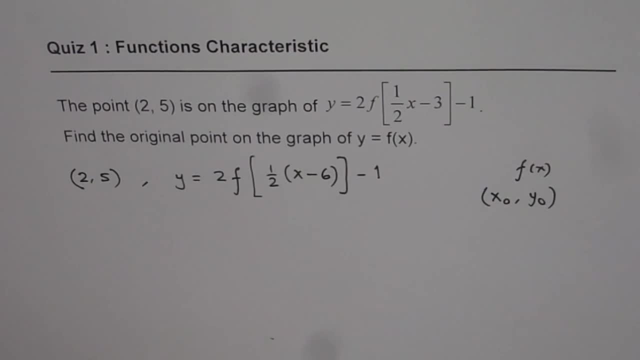 20,, 21,, 21,, 22,, 23,, 24,, 25,, 26,, 27,, 28,, 29,, 30.. Here x minus y equals to f of x is the original point on the graph. 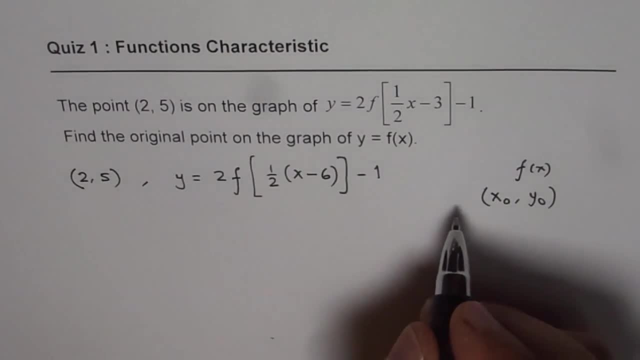 Right now the original x function of y equals to 0.. So if y is not z, then how can we find the original x function on the graph of y equals to f of x. If we need or so, then we will like to use the Tanalussi andistic trigonometric functions. 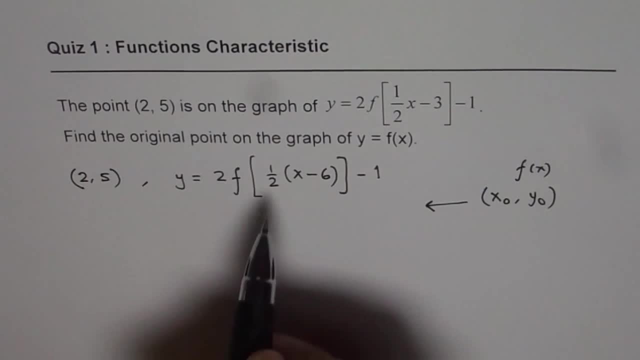 to tidy up both x and y into terms. So we need z and y and these two points. what happens now? So x1 is the point we have to find, The point we have poliv Zoom 0. It is a common word. 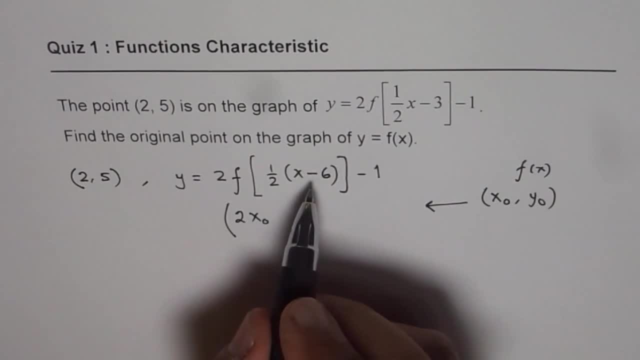 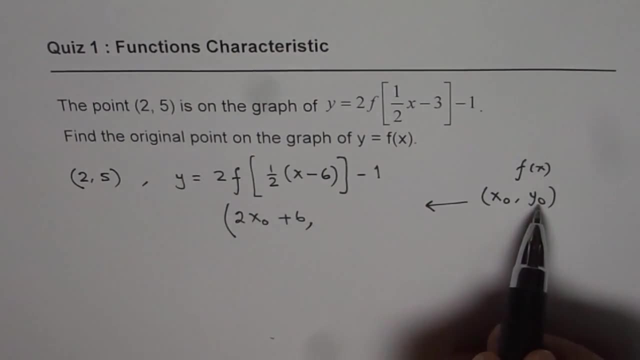 How about 10? Middle max? So x is an elementary point times x0, and then we have to add 6 to it, plus 6.. So that happens to the x value. As far as y value is concerned, it gets multiplied by 2, so it becomes 2 times y0,. take away: 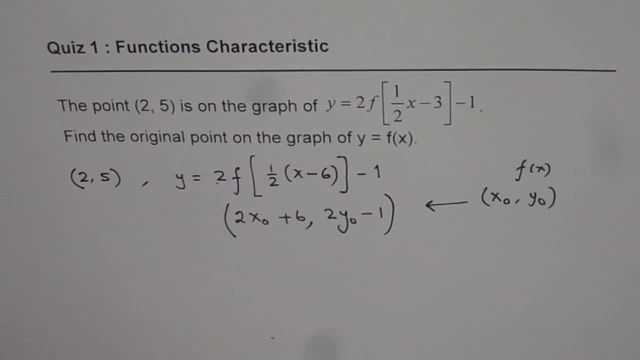 1, right. So that is the transformation. Now, here, what we are given is that 2 times x0 plus 6 is 2, right. So we have 2 times x0 plus 6 equals to 2.. From here we can find: 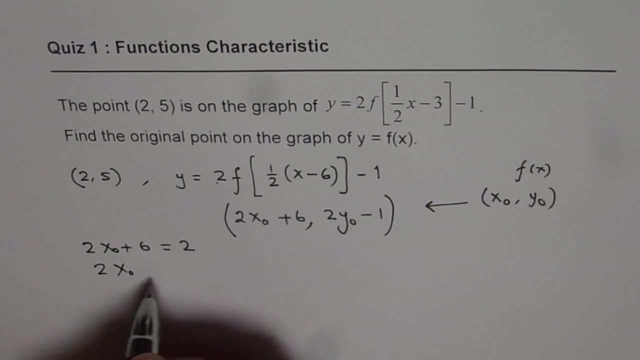 the x coordinate value, which is 2 times original value of x, should be 2 minus 6,, which is minus 4, and x0 is equals to minus 4 divided by 2, which is minus 2.. And we can find the y.